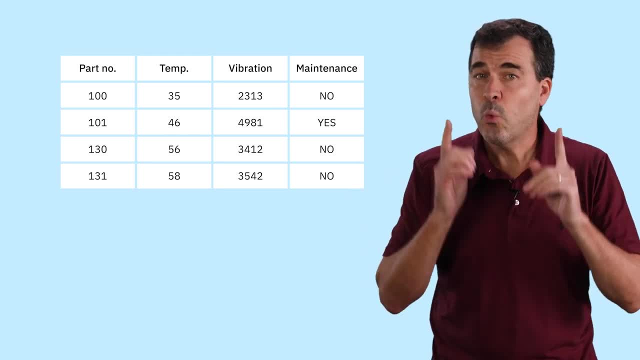 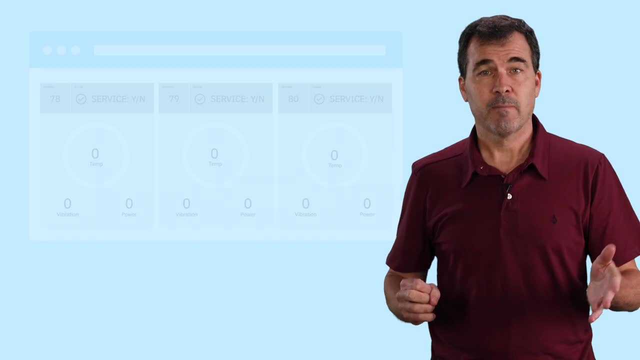 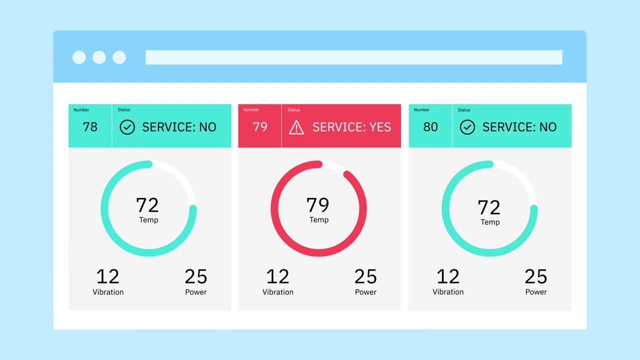 Maintenance needed, yes or no, And basically that's supervised learning. We provide labeled data and supervised learning produces a model which can accurately predict that label. Now, when the prediction is something like yes or no, maintenance needed or not needed, we call that binary classification. Then there's multi-class classification. 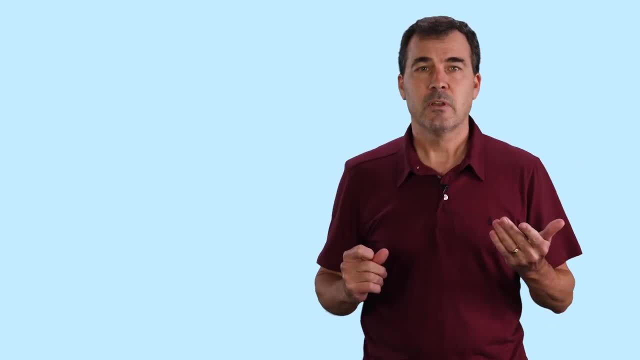 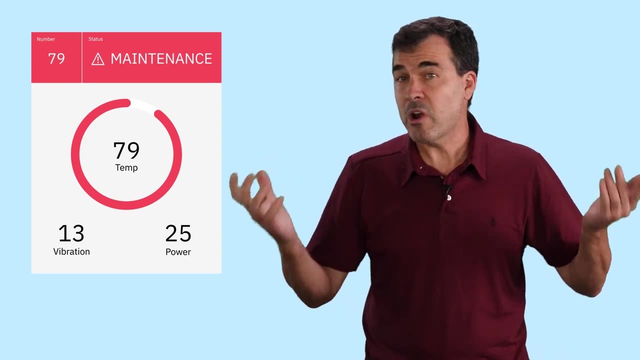 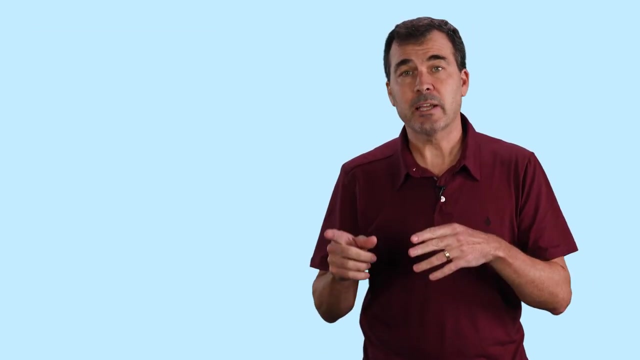 We have a tongue twister that indicates any number of states. So in our robot example, a multi-class classification might indicate if the robot needs maintenance or not, needs replacement or just needs some rest. In other words, the multi-class approach provides more context. Using our binary classification model, we were able to 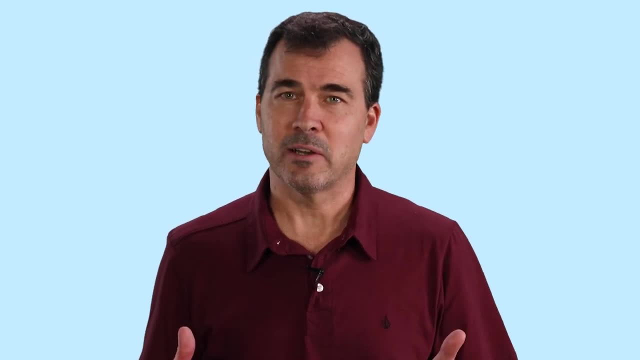 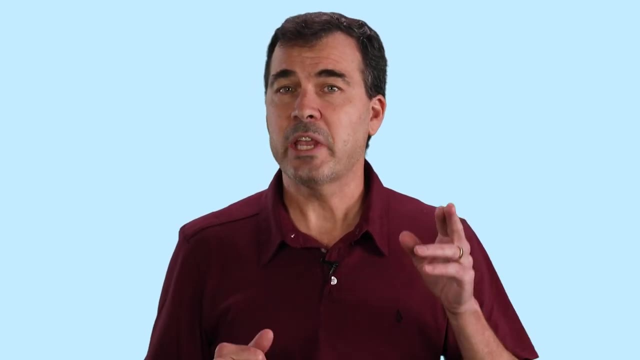 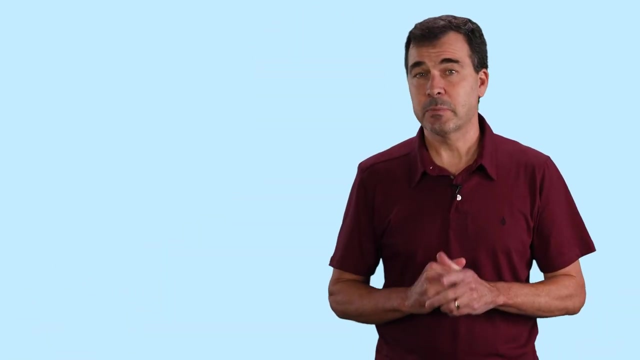 schedule maintenance on demand by feeding real-time metrics into our model and getting a simple yes or no Using the multi-class classification model. we got that and we added whether we might need a replacement robot or could just give a robot a break. Another popular form of supervised machine. 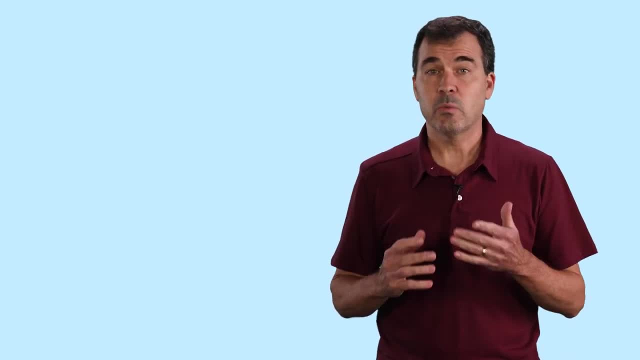 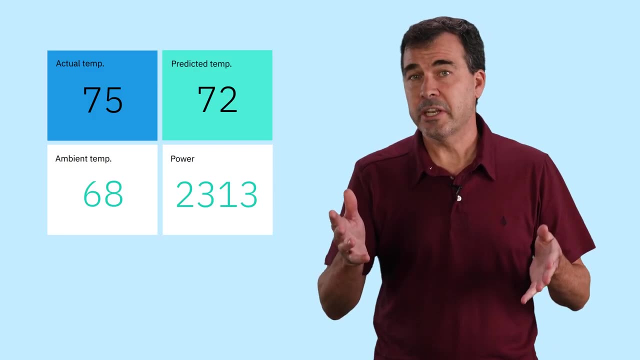 learning is called regression. Regression is used when you want to predict a continuous value like temperature. Back to our factory. We can train a model to predict what a robot's temperature should, be given how hot it is in the factory and the robot's power consumption. 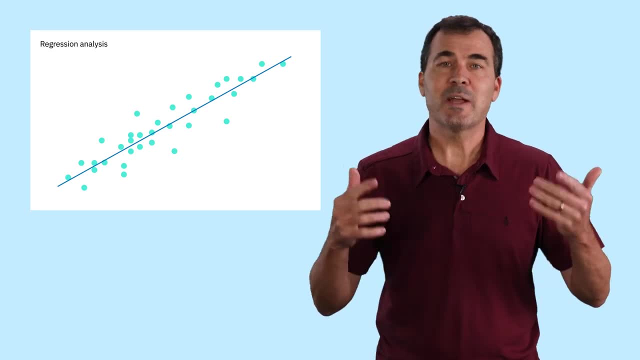 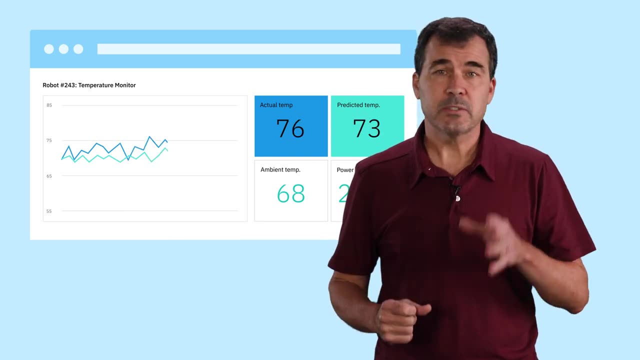 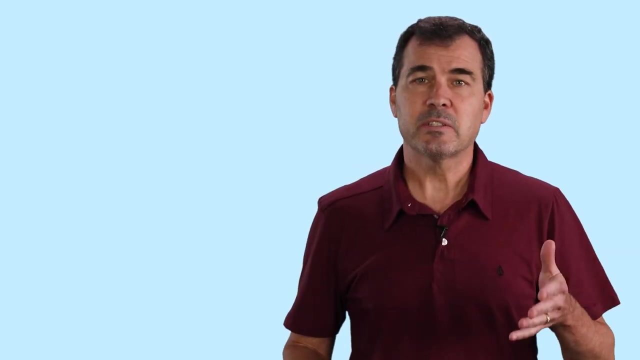 With that model, we can compare the predicted temperature to the robot's actual temperature, Unlike our first example, where we predicted maintenance needed or not. with regression, we might use a dashboard to keep an eye on the situation instead of getting a predictive yes or no. Okay, now we understand the basics of supervised 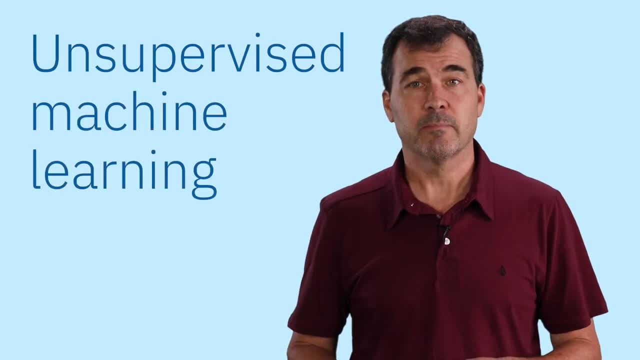 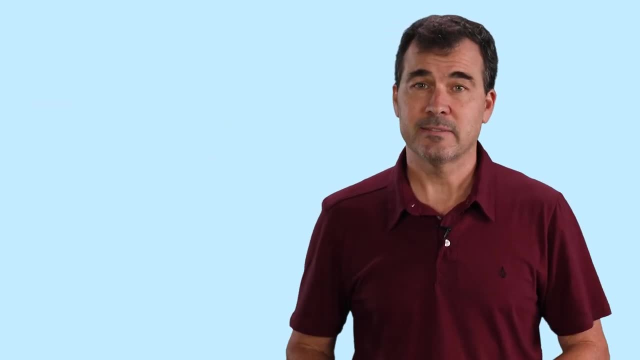 machine learning. Let's take a look at unsupervised machine learning. Remember this is the approach that learns from a data set without labels. Instead, we look for patterns in the data are three main types of unsupervised learning. The first is called clustering: which groups? 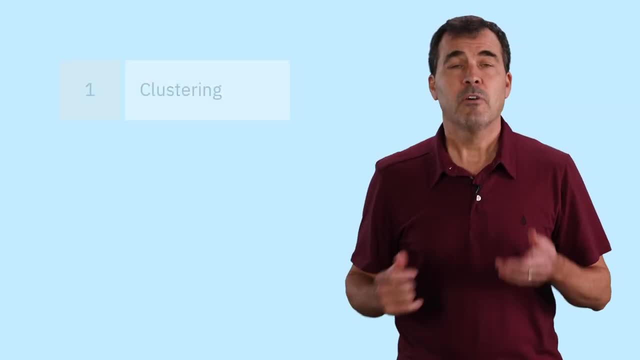 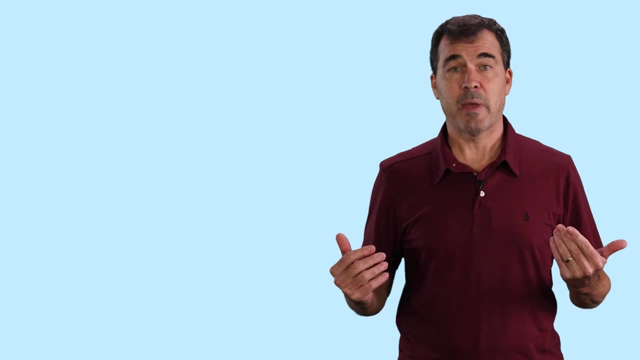 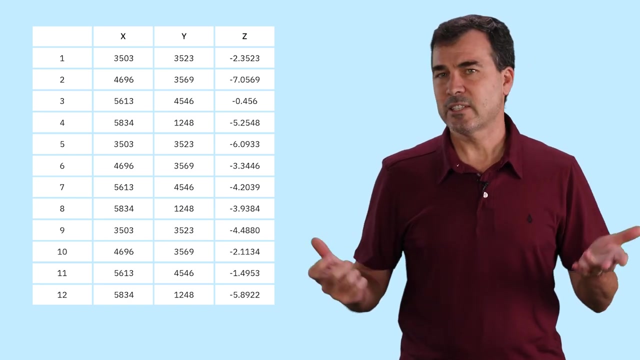 unlabeled data based on similar characteristics. For example, an online store might use clustering to develop customer personas that group people with similar buying patterns. So how is clustering helpful? Well, take a look at this dataset. Even though this is relatively small, it's. 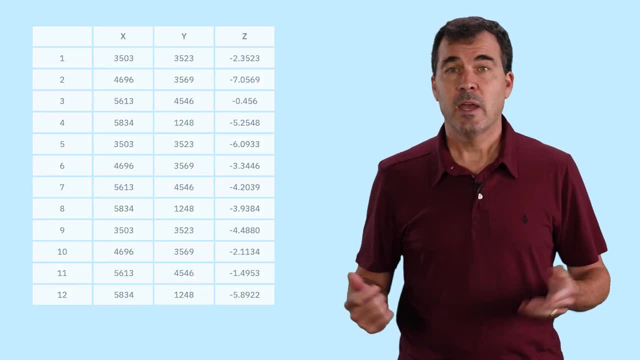 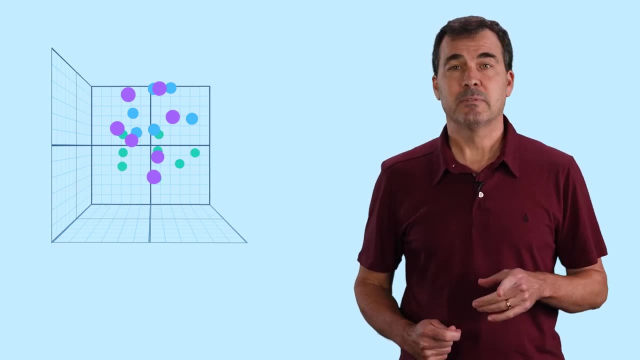 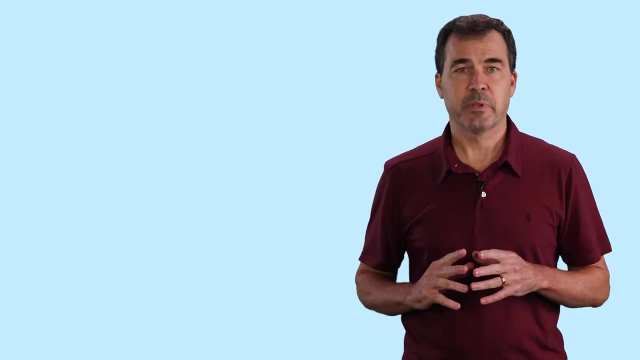 still hard for the human eye to detect any patterns. Now look at this image we produced with clustering In this 3D diagram. we've plotted out the numbers in that table. Now we can easily see clusters or spot any outliers. This has major implications for online retailers. 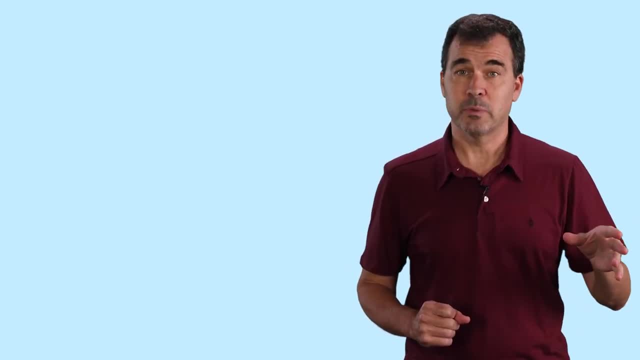 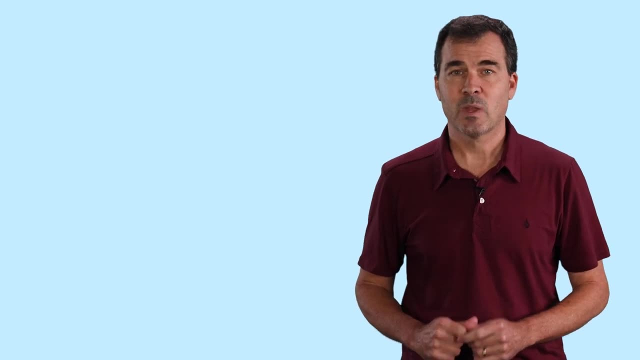 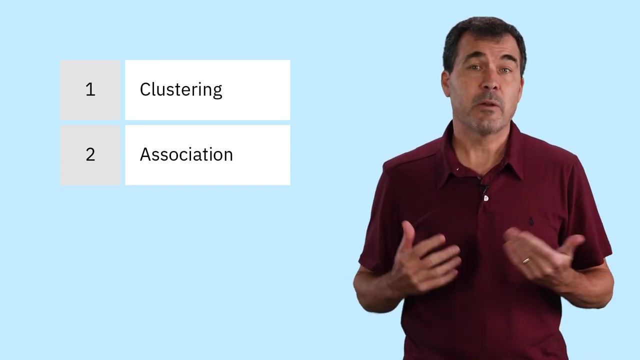 Using this model, you can tailor your user experience for each group. You can also flag customer behavior that doesn't fit any persona and could be identity fraud. The next type of unsupervised machine learning is called association. Association is used to identify relationships. 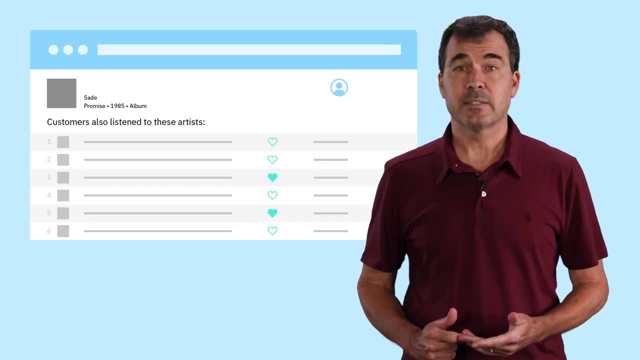 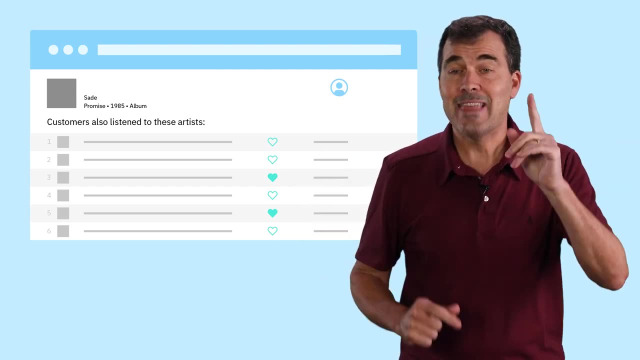 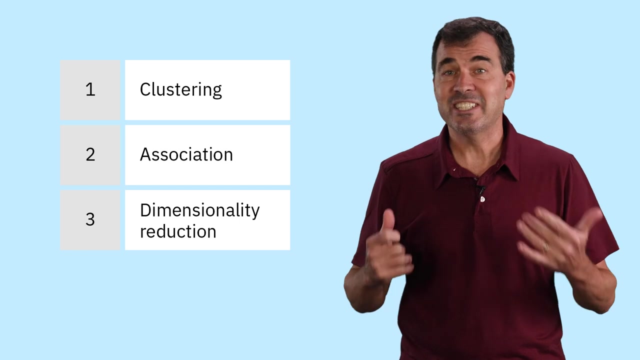 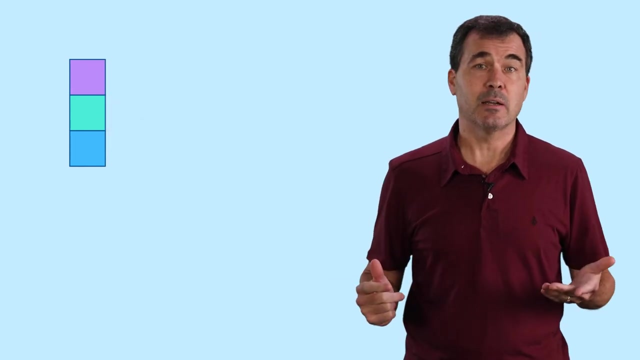 in the data. Picture your music streaming playlist When your platform pops up a message: people who liked X also liked Y. That's association. Finally, there's dimensionality reduction. It helps eliminate noisy, redundant data from unmanageable datasets. This reduction simplifies the input data before training a model. It's. 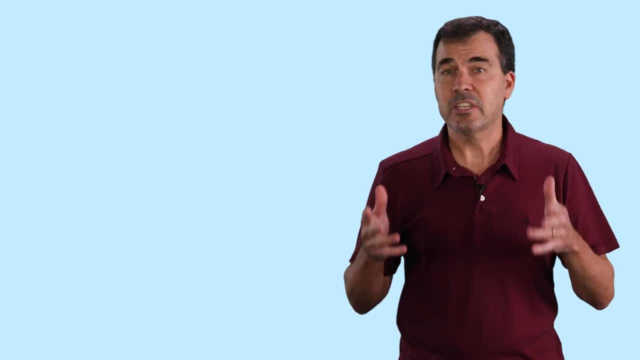 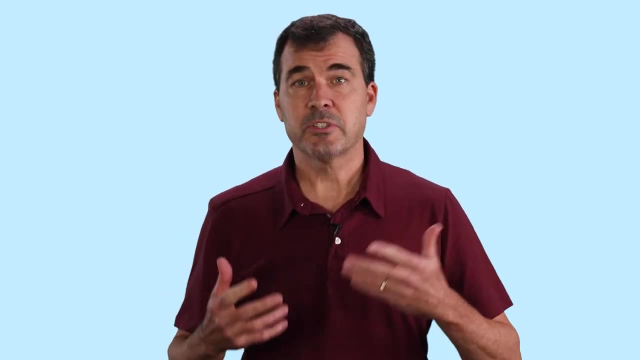 sort of a smart, customer friendly relationship for deaf interpretive users When creating tactical way to trim fat and actually get more accurate results with less data. Okay, so that's my brief overview of supervised versus unsupervised machine learning, But the question remains: 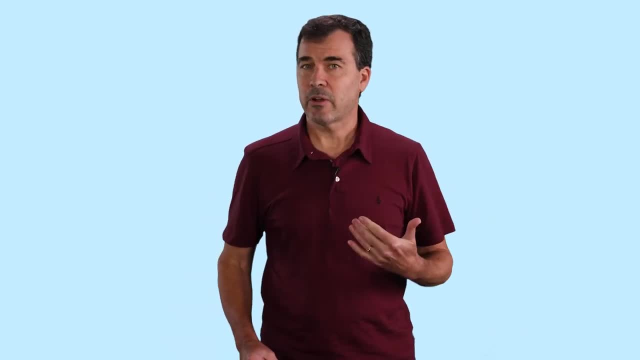 which approach is right for you. If you want to predict outcomes and you're willing to train your model by manually labeling your data, supervised learning is your best bet In our factory example: knowing what robots needed servicing reduced downtime with proactive and cost-effective maintenance. But if you have lots of data and are struggling, 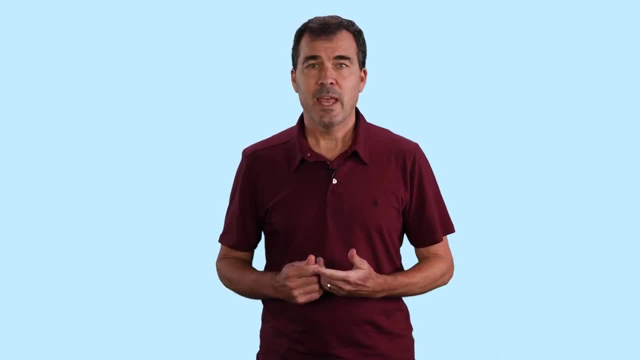 to identify patterns go with unsupervised learning. It can help clear the fog that's preventing you from seeing what the data is telling you. In our simple music shopping example, grouping shared interests helped improve the customer experience and boosted sales. When you're ready to start, think of it as an experiment. 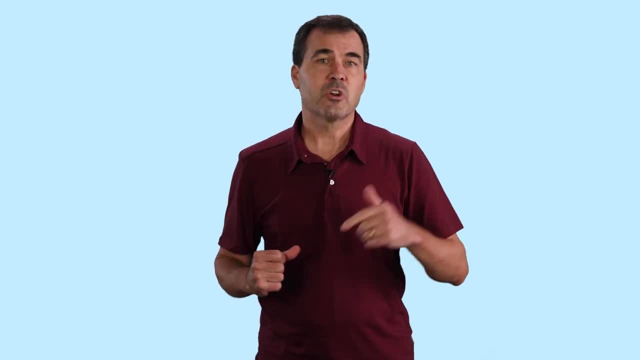 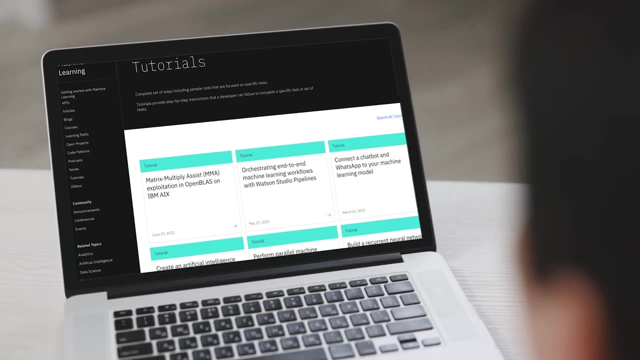 There are many different tools you can try. Check out the links in the description to get started. If you want more information on machine learning, check out the link in the description to get started. If you like this video and you want to see more, please like and subscribe. If you have any questions, drop them in the comments below.